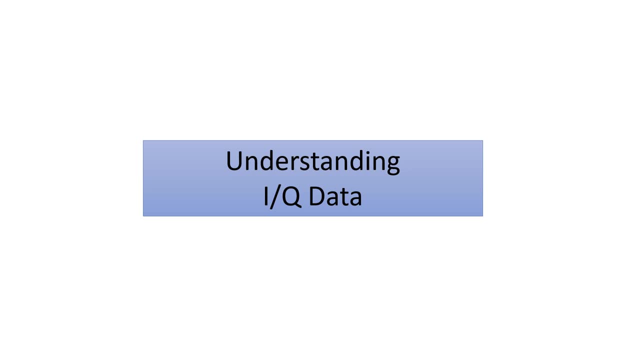 All right, folks, today we're going to give a simple talk on IQ data. IQ data is heavily used in all your software-defined radios out there. Any kind of digital communications radar, sonar, radio, astronomy- all that is going to have some. 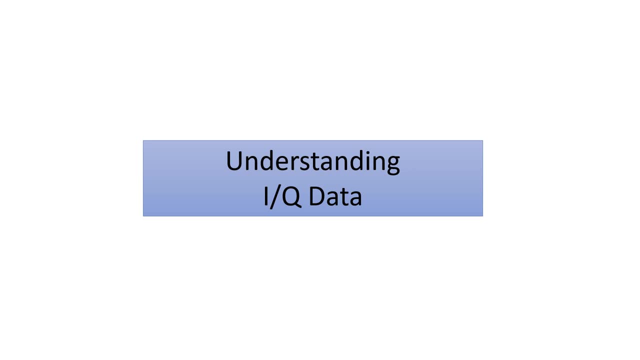 kind of IQ data that you need to process. So let's get into, let's just say, a motivation for it or why we would want an IQ demodulator. So let's take our example here We have a local oscillator at 180 megahertz. We have an incoming 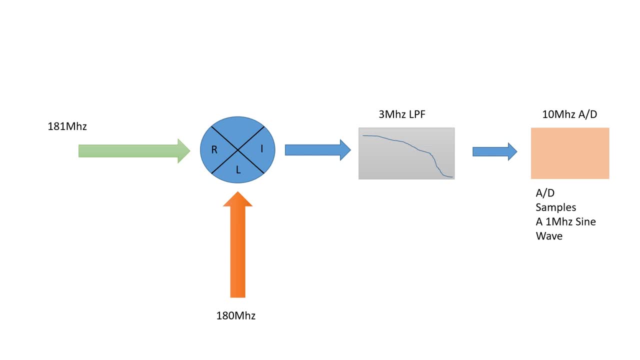 signal at 181.. This is going through a mixer- For our purposes, let's just say ideal multiplier- such that the product is only going to be the sum and difference of these two guys. We low-pass filter it so that we only are picking. 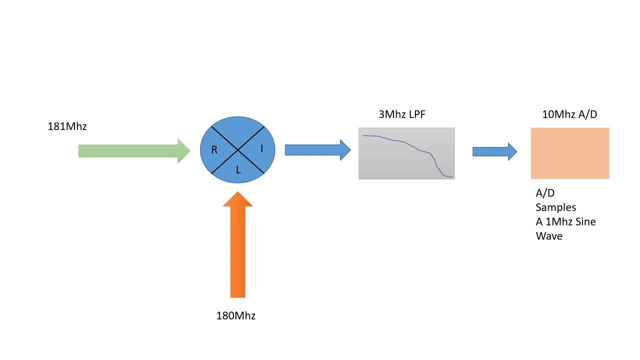 off the difference frequency and it's clear that this 80D analog-to-digital converter running at a 10 meg clock will only see a 1 megahertz sine wave right, Because the difference between 181 and 180 is 1 megahertz. 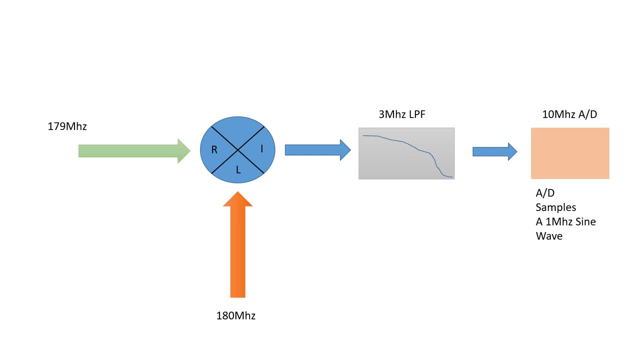 So far, so good. but now let's say the input signal is 179.. Well, the analog-to-digital converter over here will also see 1 megahertz. Some might say it's a negative 1, but the analog-to-digital converter will not be able to tell that. 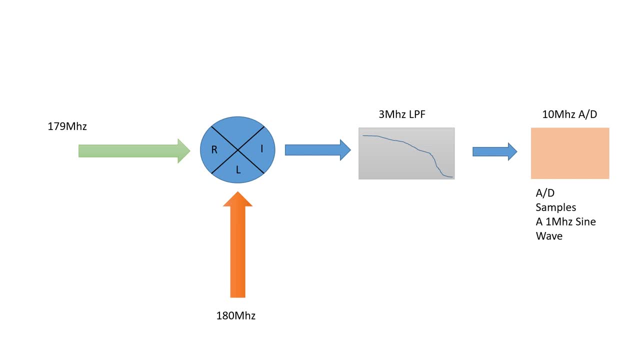 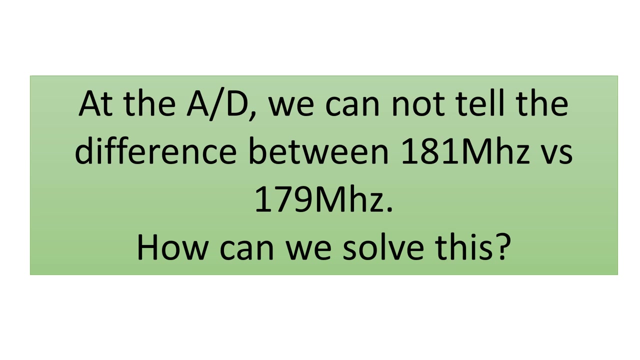 because it only has 180D. It does nothing to reference to it or compare it. So in terms of at the 80D here we cannot tell whether basically 179 is the input frequency or 181, and so basically with this current design, as I said, we cannot tell whether the signal 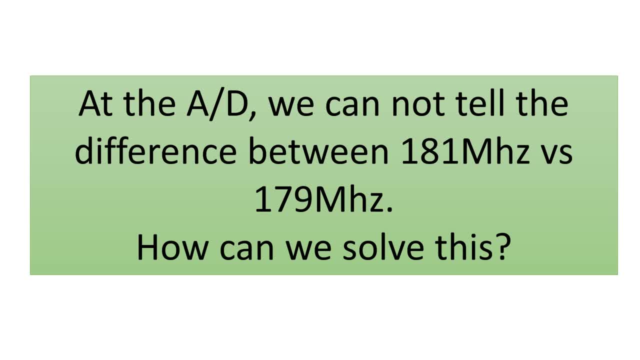 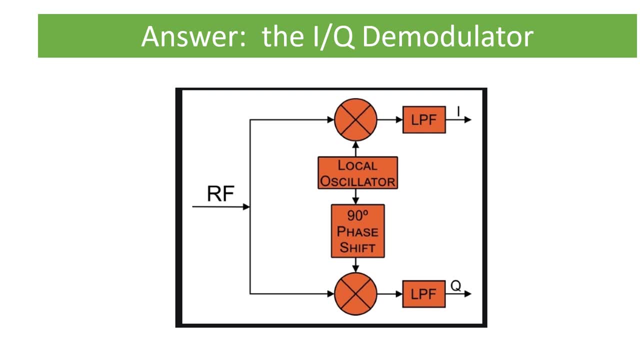 coming in was 181 or 179. so how can we solve this? answer is to implement a IQ demodulator, and this is the high level here. the RF comes in, it gets split, essentially goes to two mixers and the local oscillator is generating a cosine. 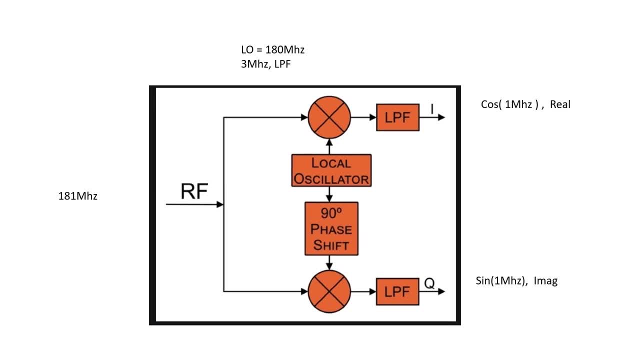 signal and a sine signal. all right, so now let's go through our example. 181 comes in again. the LO down here is set to 180 megahertz, so the I port will have the cosine of 1 megahertz, the Q port, we will have the sine of 1 megahertz. all right, so far, so good. now 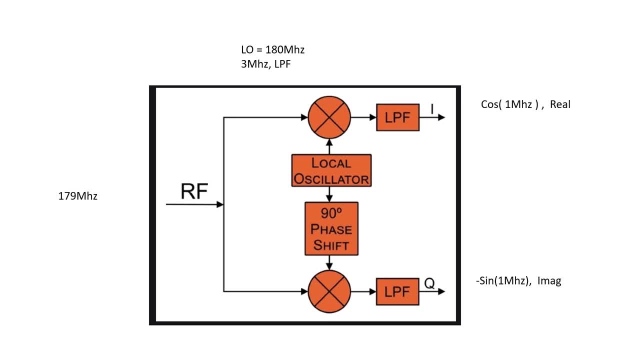 179 comes in, the I port will be the cosine of 1 megahertz. the Q port will be the negative sign. so I think it's clear now that now we have an ability to determine whether the input frequency is either below, above or below the LO. 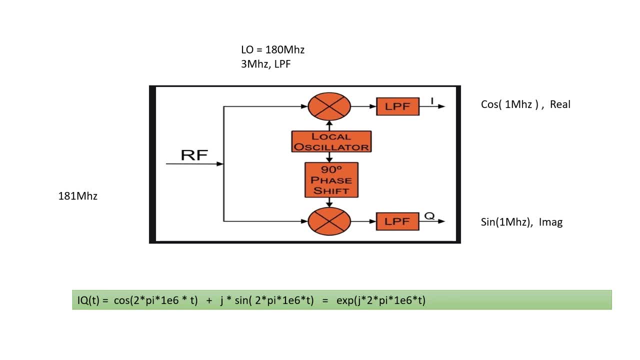 and here's the, the math for this right. so if 181 is the input frequency, the LO is 180. again, the I is the cosine, the Q is the sign. this is held down here. you express it mathematically and, and typically it's expressed in this compact. 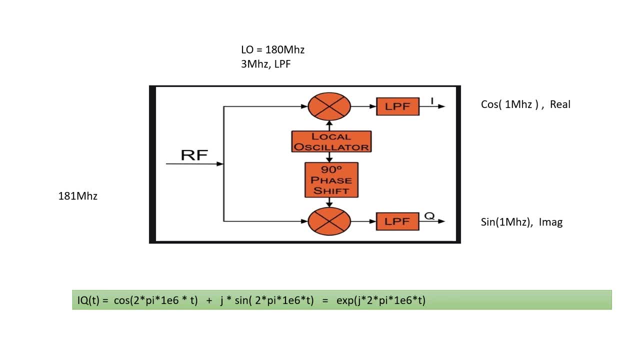 form, so this is a positive에도. the J 2 pi 1 megahertz times time for the 179 case. it's in e zer 179iecallexan E in ontograph E1 of the ohh at 00megahertz time for the 179 case it's an EUNA 1 megahertz times time for a 179 case it's an EUNA 2. of the j 2 pi 1 megahertz times time for the 179 case, it's an EUNA 15 micro motherfucker. amortization is a ع in our今天. 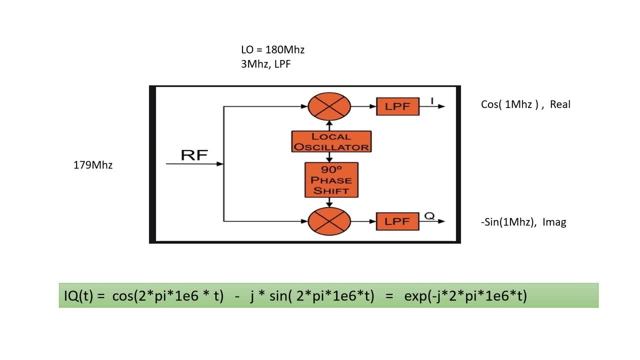 to the negative j 2 pi, 1 megahertz times time to indicate that it's going to be a negative 1 megahertz frequency, in that it's 1 megahertz below the oscillator. okay, that's, that's what we mean by negative frequencies. it now lets us know it's 1 megahertz below the oscillator frequency. 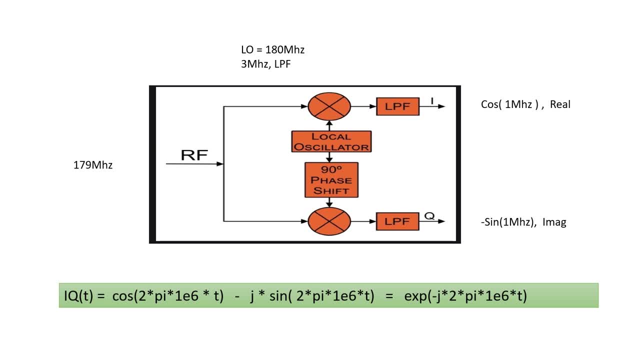 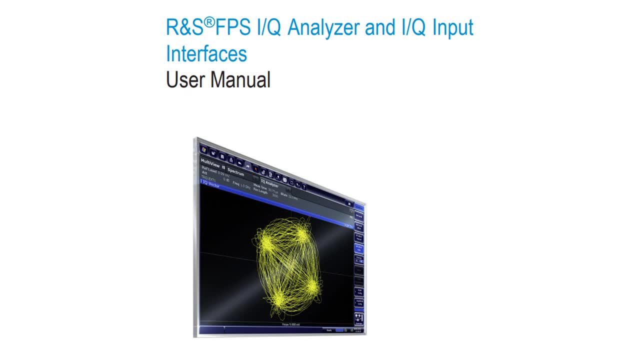 and we can do that because we have essentially an i and q to compare it to. so this is not just a magical thing. many spectrum analyzers have iq analyzer pages here that let us see the actual i and q signals. and here is one for the, the rhodes spectrum analyzer. 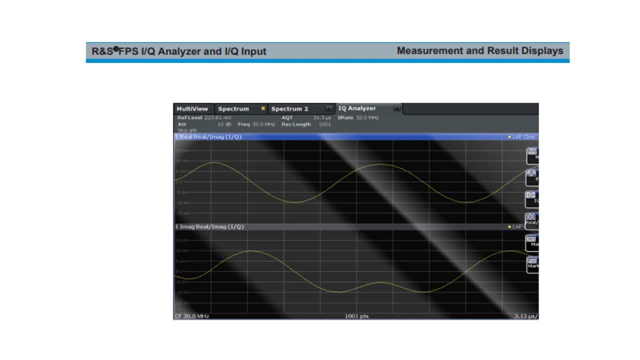 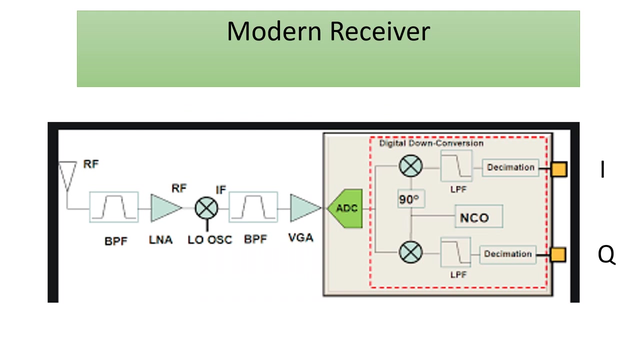 here's the i trace. the bottom is the q trace. so again, this is just showing you guys, this is not just some mathematical white paper- that this really is real signals that we can look at with modern equipment. so this would be a typical example of a modern receiver. the rf comes in. it's somewhat bandpass, filtered, amplified. there's an. 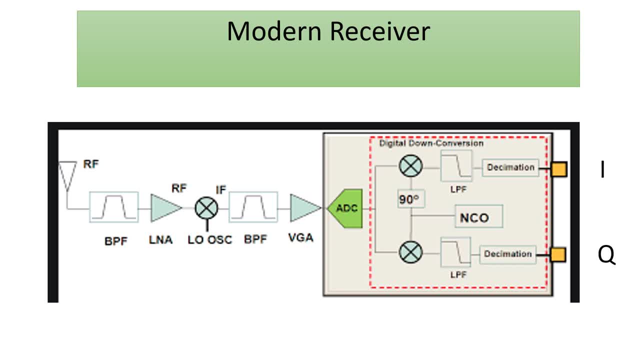 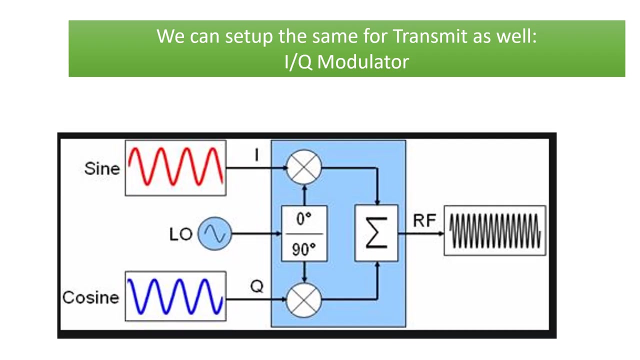 local oscillator that mixes it down to some center if frequency, and then that if frequency is digitized and converted to what is essentially called baseband iq- and this is the i and q data- that would go down to get further processed. so we've talked about iq demodulators, but we can also do the same thing for transmit. 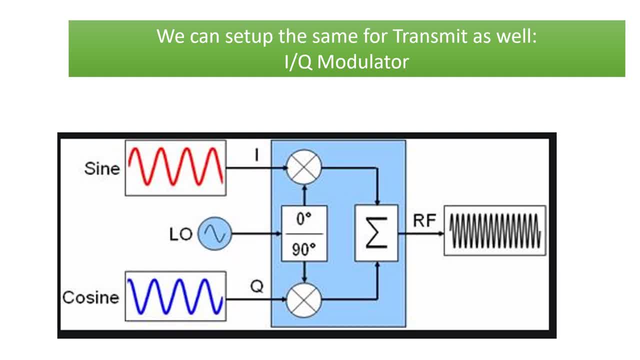 obviously that would be called an iq modulator. it's the same idea, basically in reverse. you have the lo, which is the center frequency of where you want to transmit, and you feed this thing an i and q signal, and you can also do the same thing for transmit. 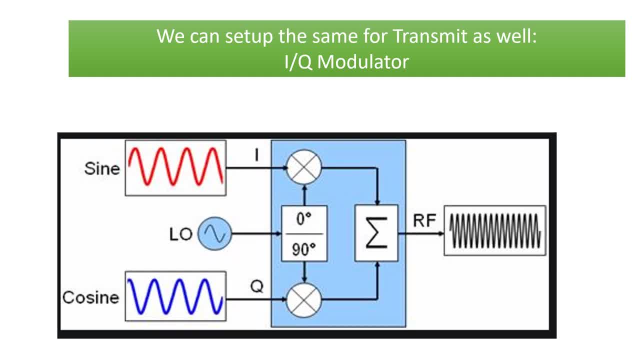 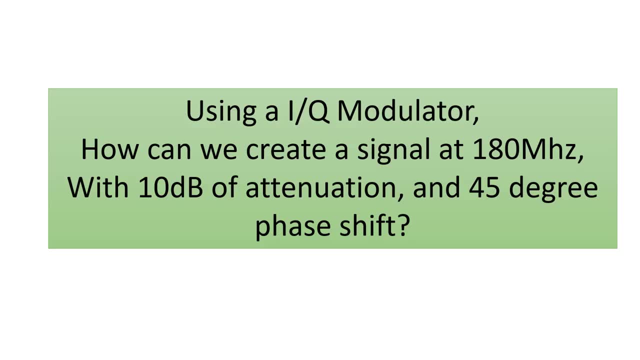 signals to create the final rf signal. so this i and q are baseband signals and the lo here is what's basically being the carrier of the final frequency we want to come out. so let's just go right into an example. so let's just say we want to create a signal. 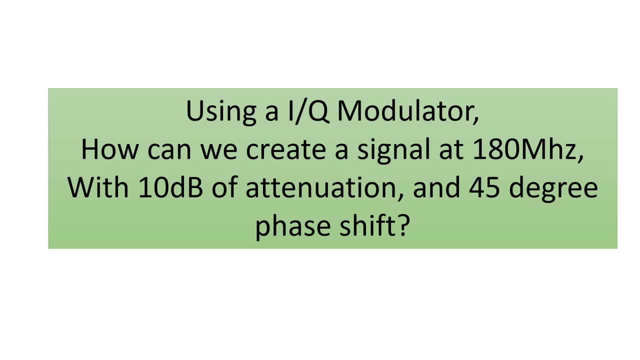 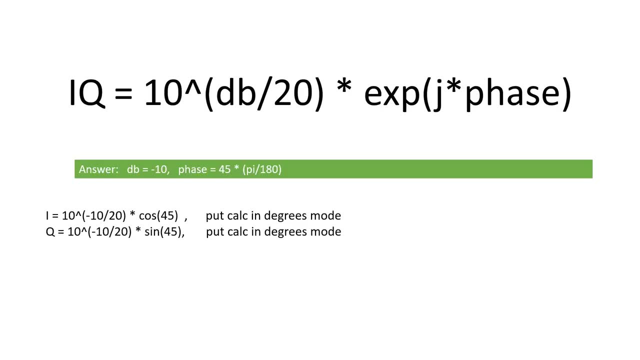 at 180 megahertz and we want to apply 10 db of attenuation and give 45 degree phase shift. here's the equation of how we do that and here's explicitly how we break out the i and q numbers. so chug those in your calculator and that's the i and q numbers that, if you 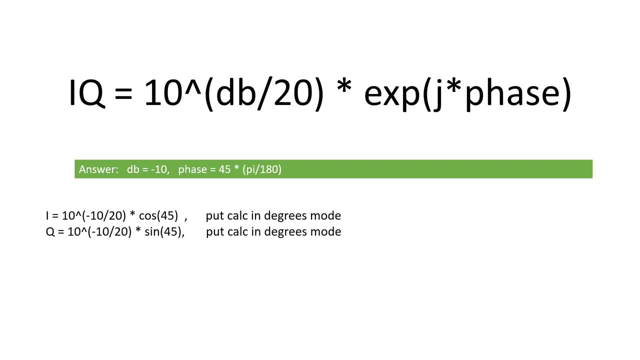 presented to a iq modulator, it would attenuate to signal by 10 and put a 45 degree phase shift. so this is one way how you can start representing digital bits. basically, every bit will have a unique phase and attenuation. they call it a fancy name, like quam 64, but it's basically using this equation you're representing all your